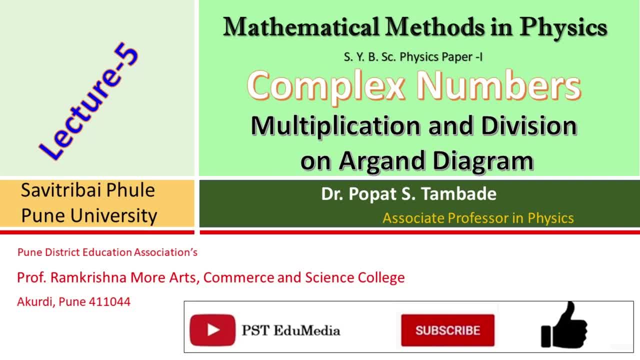 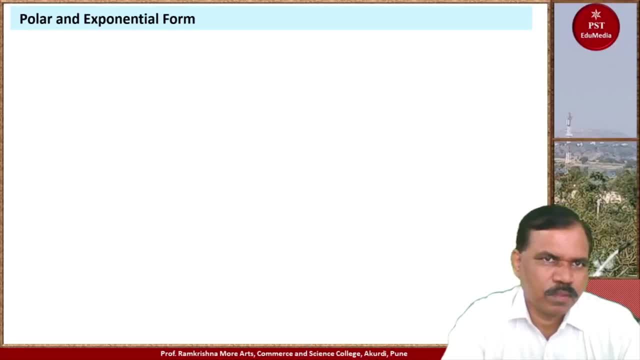 Hello students, Welcome to video lecture on complex numbers. In this video lecture I am going to discuss about multiplication of complex numbers on Argonne diagram and division of complex numbers on Argonne diagram. We have already seen polar and exponential form of the complex number. We will revise that. 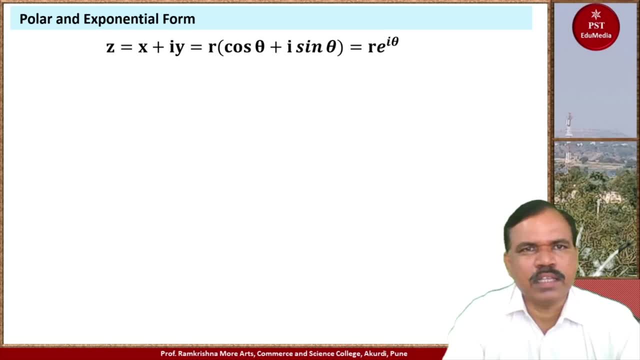 So suppose z is equal to x plus iy, we can write it in polar form as: r in bracket, cos theta plus i sin theta. where theta is argument of the complex number and r is modulus. In exponential form we write it as r e raised to i theta. 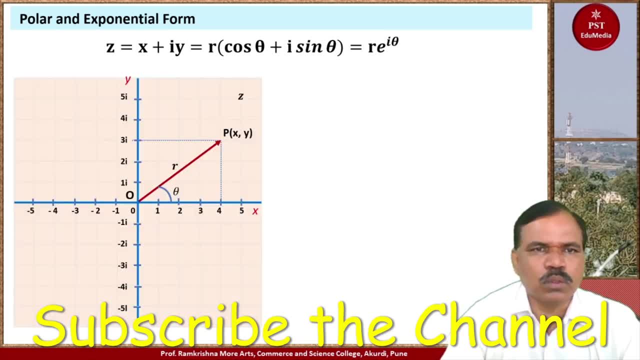 And graphically it is represented So that op line or op vector represents complex number z on xy plane, and x is real part and y is imaginary part. r is modulus of z and this theta is called argument of z. So we have seen this already. 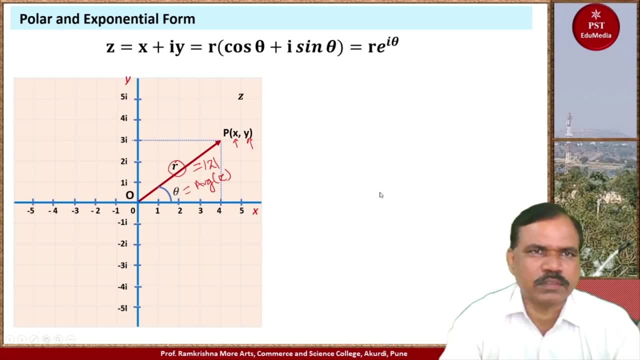 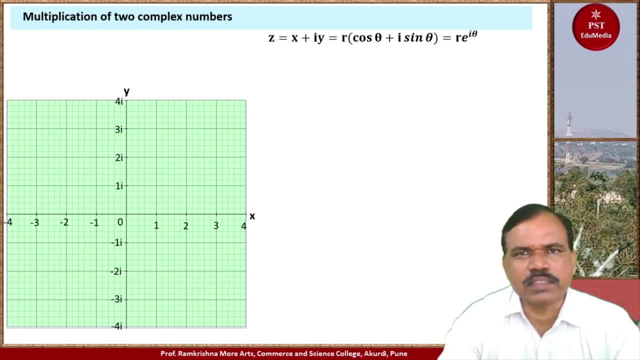 Now we will go to multiplication of complex numbers. So suppose we know in general z is equal to x plus iy is equal to r in bracket cos theta plus i, sin theta and it is equal to r e raised to i theta in exponential form. 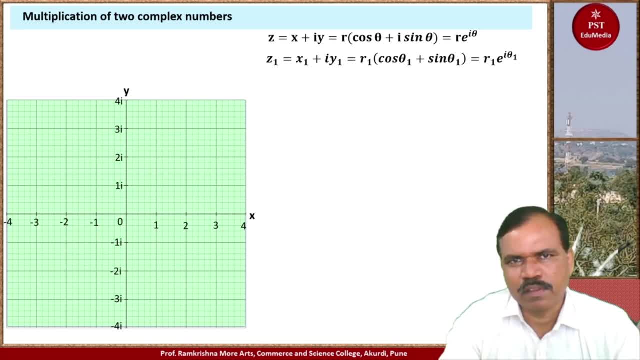 Suppose we have first complex number z1, that is equal to x1 plus iy1, in rectangular form, which is equal to r1, in bracket cos theta1 plus i plus here i sin theta1, which is equal to r1, e raised to i theta1. 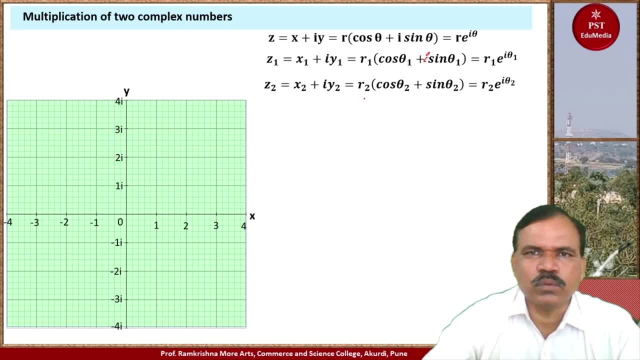 and z2 is equal to x2 plus iy2 is equal to r2. in bracket cos theta2 plus plus i, sin theta2 is equal to r2, e raised to i theta2.. So these are exponential quarks. Now here first complex number. 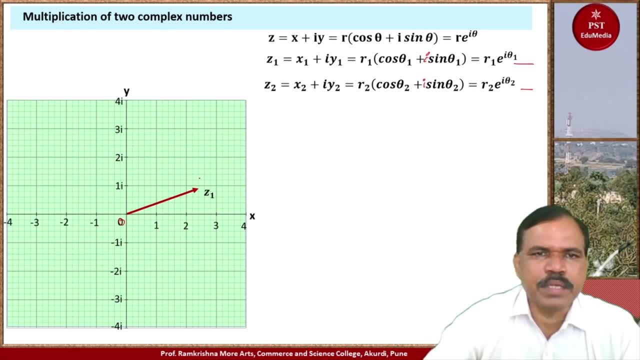 it is represented by vector op on Ergun diagram. Its modulus is r1 and argument is theta1.. If we take z2, it is represented by oq- vector oq on Ergun diagram, with modulus r2 and argument theta2.. Now, if we take product of two complex numbers, 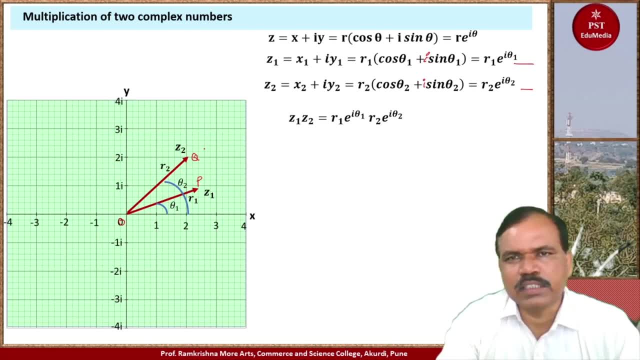 z1 into z2.. That is r1, e raised to i, theta 1, into r2, e raised to i, theta 2.. So we can write this: as z is equal to z1 into z2, which is equal to r1, r2 into e raised to i, in bracket theta 1 plus theta 2.. 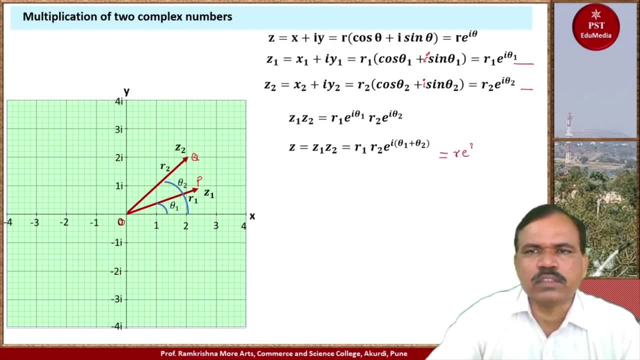 So we can call this as r e raised to i theta. So r is modulus of this z and theta is argument of this z. So here this z is represented by or, and its magnitude is r1 into r2 and argument is theta 1 plus theta 2.. 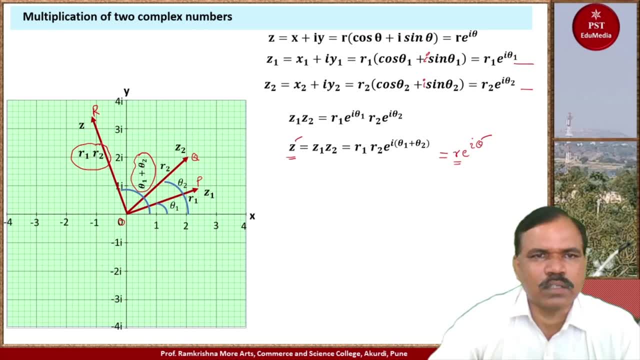 Theta 1 plus theta 2 and modulus is r1 into r2.. So when two complex numbers are multiplied, their arguments are added, So argument of z1 into z2.. So z1 is equal to argument of z1 plus argument of z2.. 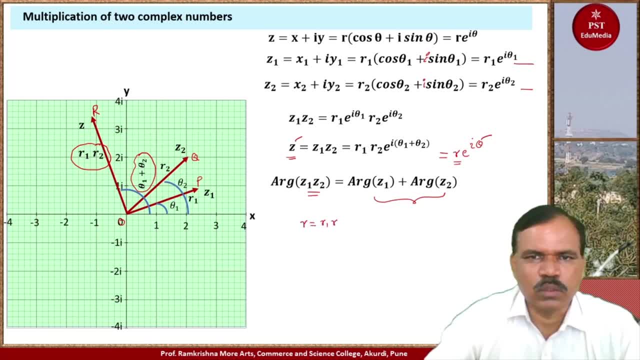 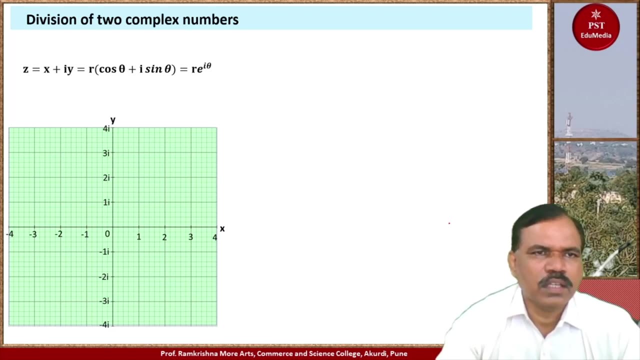 And r is equal to r1 into r2.. That is, modulus of z will be equal to modulus of z1 into modulus of z2.. Now we will go to division of two complex numbers. Here we have: z is equal to x plus iy. 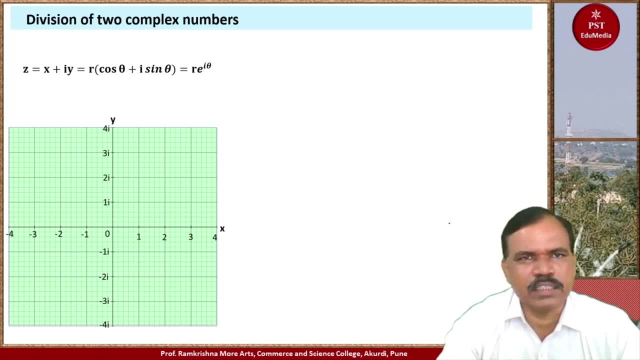 That is equal to r. in bracket cos theta plus i sin theta, That is r. E raised to i theta. Now let us take two complex numbers: z1, that is x1 plus iy1, which is equal to r1. in bracket cos theta 1 plus i sin theta 1.. 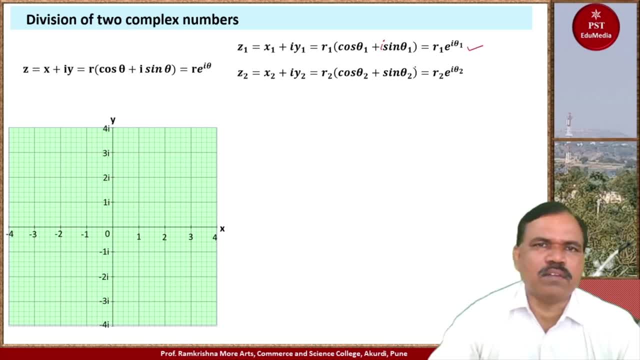 Which is equal to r1 e raised to i theta 1.. And z2 is equal to x2 plus iy2, which is equal to r2 in bracket cos theta 2 plus sin theta 2., Which is equal to r2 e raised to i theta 2.. 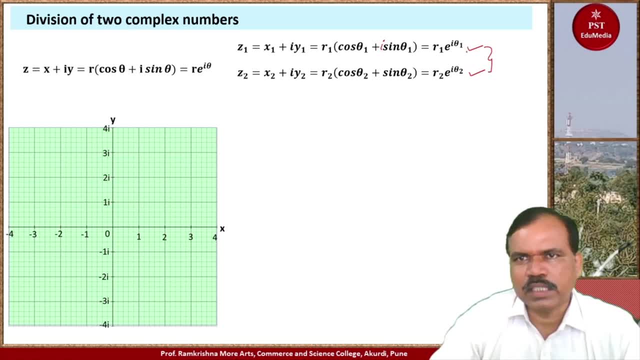 So these are the two complex numbers, These are exponential forms. These two Theta 1 and theta 2 are arguments of z1 and z2 respectively. Now, if we take division, z1 upon z2 is equal to r1. e raised to i, theta 1 upon r2, e raised to i, theta 2.. 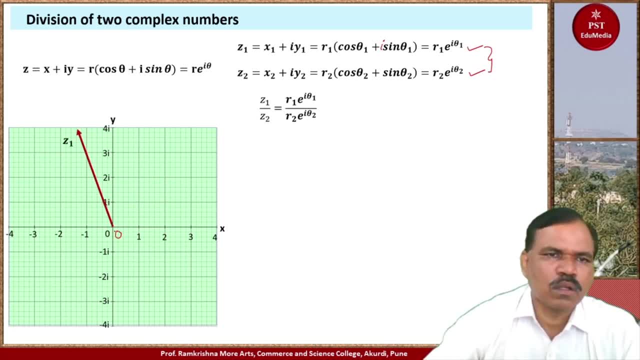 So z1 is represented by op on argon diagram With modulus r1 and argument theta 1.. Now z2. it is represented by oq vector, oq on argon diagram With modulus r2 and argument theta 2.. Now z1 and z2.. 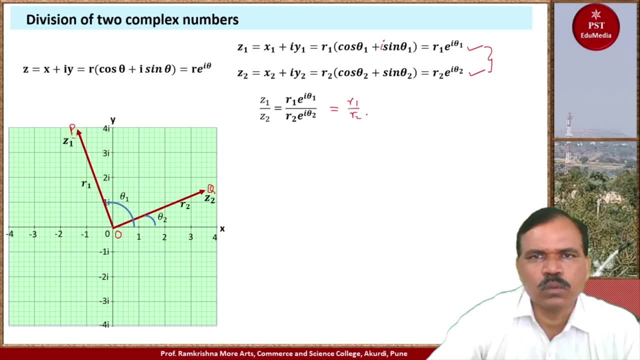 So we can take this as r1- r2.. r1 upon r2 into e raised to i theta 1, into e raised to minus i theta 2.. So here Here we get z is equal to z1 upon z2, which is equal to r1 upon r2, into e raised to i in bracket: theta 1 minus theta 2.. 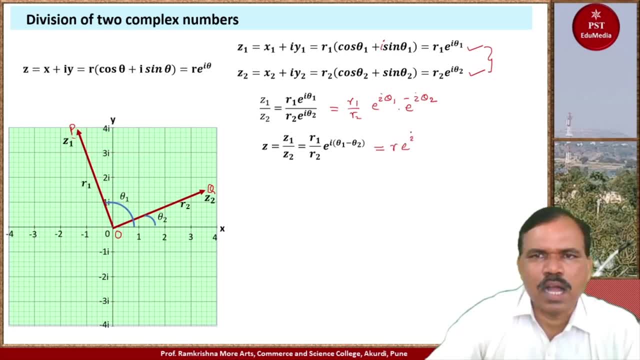 So we can write this as r e raised to i theta, where r is equal to r1 upon r2 and theta is equal to theta 1 minus theta 2.. So this z, it is represented by o r On the argon diagram, with argument theta 1 minus theta 2 and modulus r1 upon r2.. 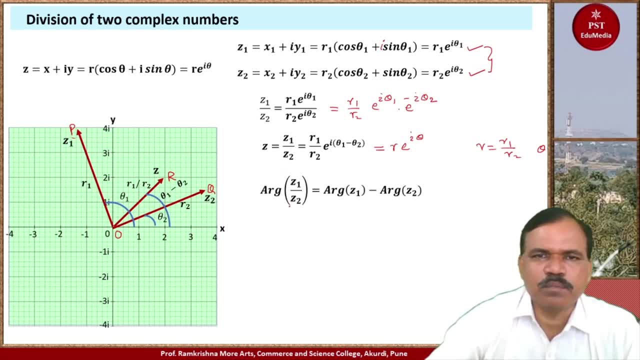 So if we see here argument of z1 upon z2, it is equal to argument z1 minus argument z2.. So when complex numbers are divided, their arguments are subtracted. So this is about division of two complex numbers on argon diagram. Now let us go to simple example. 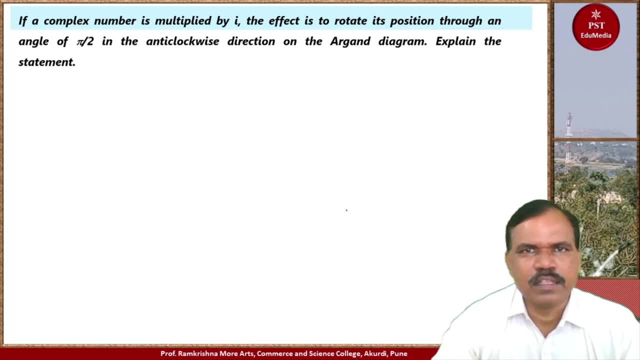 If a complex number is multiplied by i, The effect is to rotate its position through an angle of pi by 2 in clockwise direction on the argon diagram. Explain the statement Means: suppose we have complex number Like this: Z is equal to x plus iy. 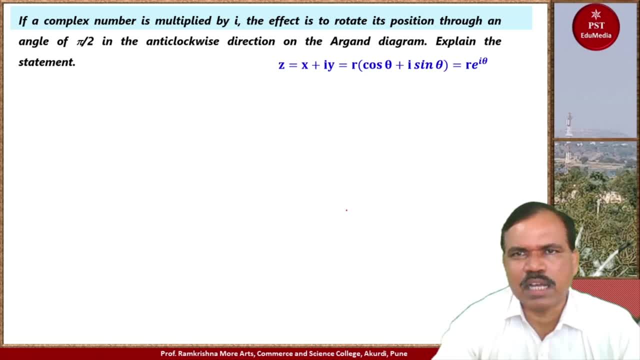 Which is equal to r in bracket cos theta plus i sin. theta In Polar form is equal to r, e raised to i theta, And we know on argon diagram it is Represented by vector op. So theta is argument r is: 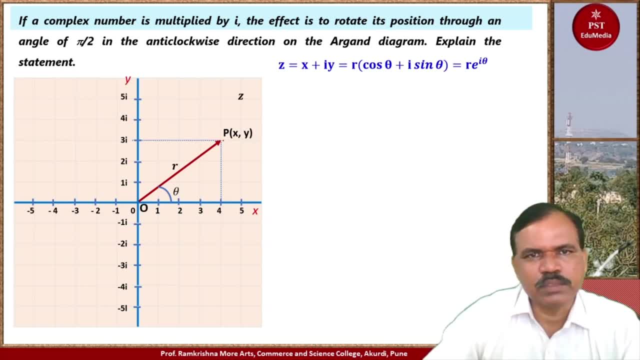 Modulus of the complex number And p is point representing the complex number on z plane or argon diagram. Now what is given in the statement? If a complex number is multiplied by i, The effect is to rotate Its position through an angle of pi by 2.. 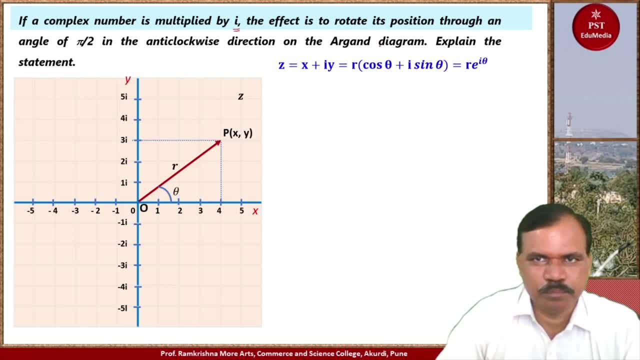 In the anticlockwise direction on the argon diagram Means angle increases. Explain the statement: So z is equal to x plus iy, So we will write i, z. So i is multiplied by z. Now we know Z1 into z2.. 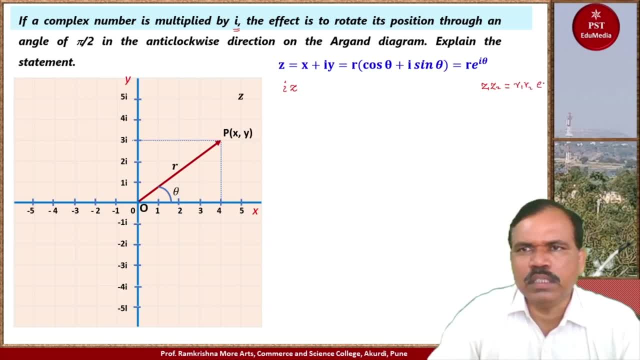 Is equal to r1 into r2.. E raised to I theta: 1 plus theta 2.. We know this. So we have two complex numbers here: I and z. Now z we have taken R, e raised to i theta. 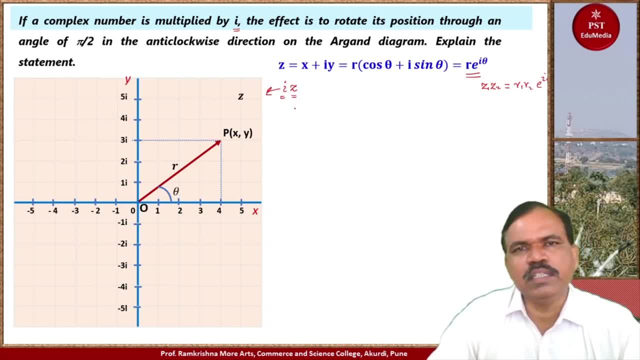 Now we will Find polar form of the complex number i. So let us call this as z dash. So z dash is equal to i, So I can write this as 0 plus i. So here X is equal to 0.. 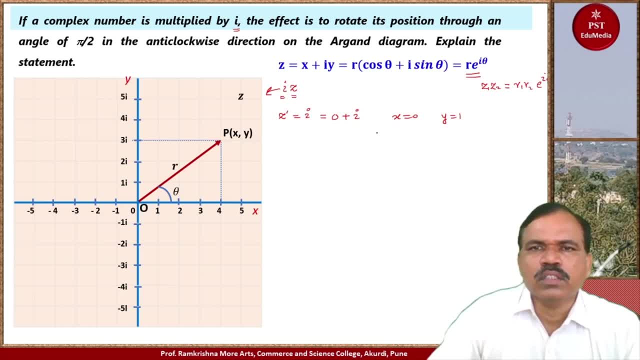 Y is equal to 1.. So here R is equal to root of X square plus y square. I will call this as r dash, That is 0 square plus 1 square, So this is 1.. R dash is 1.. 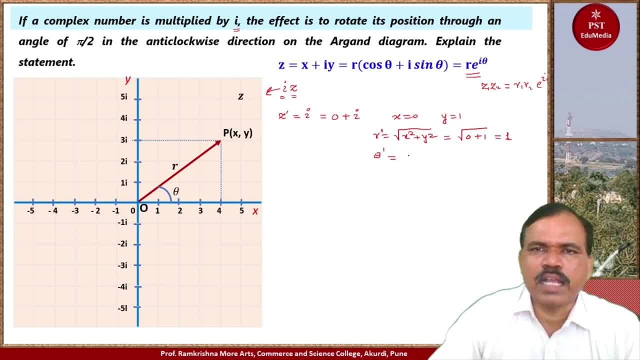 And theta dash argument. We can write this as tan inverse Y by X, Now Tan inverse 1 upon 0. So that is tan inverse Infinity. So theta dash Is equal to infinite. So I into z. 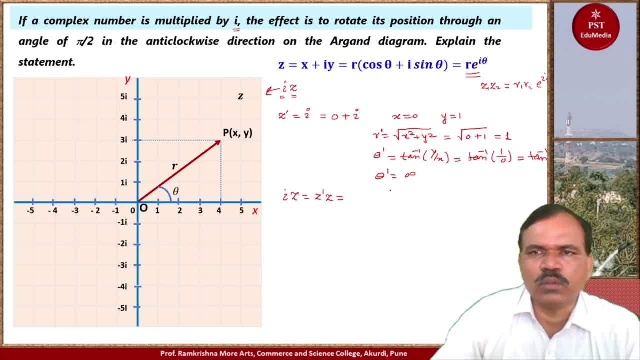 That is z dash into z Is equal to Now, it is z dash. Exponential form is 1 into e R. Theta is Pi by 2.. Not infinity Pi by 2.. Pi by 2.. So z dash into z.